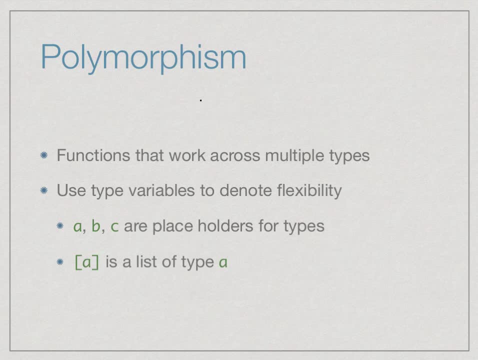 multiple input types like this. so we would like reverse, for instance, to work on lists of int or lists of float or even lists of lists, so long as the underlying value is a uniform type. so in Haskell we use type of the box and so on. so it would be nice if we could assign within the type system that Haskell 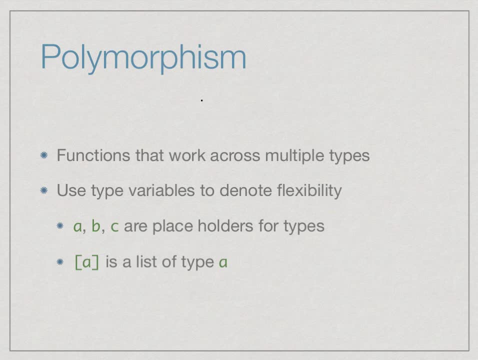 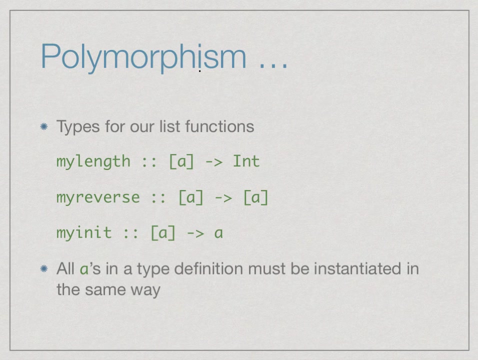 variables- usually ABC letters like these as placeholders for type. so if we say that a function takes as input type a, it means a can stand for any input. and if a stand for any input, then if you put square brackets around a, then we denote a list of that type. so if we go back now to our list functions, what does my 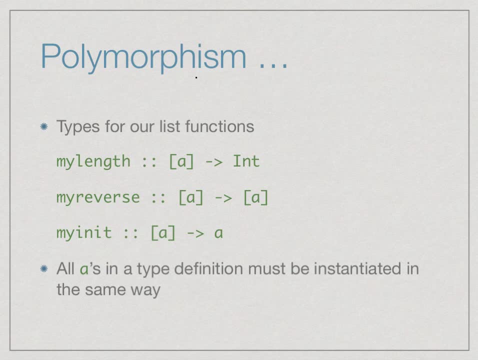 length do my length? takes any list and produces the length. the length is a number, so the output type is int. the input type is unconstrained. it can be a list of any type of a, so we write the type as list to int. Reverse, on the other hand, takes a list and produces another list, so once again it takes an. 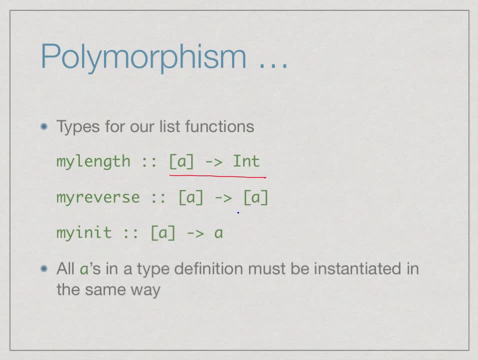 arbitrary list, but it produces a list of the same type. so it's important that the a on the left and the a on the the right are actually the same a. it means that if I give it an input of list of int, it will produce an output which is a list of int. if I give it a list of 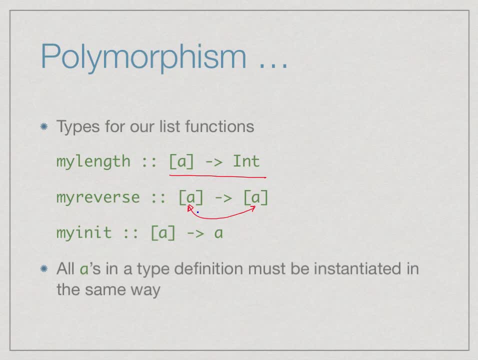 float, it will produce a list of float as output. you cannot change the type, but the type itself is not fixed in advance. and finally, if you look at my init right. so what it does is it actually produces, so there's a small mistake here. so it takes again a list of a and produces a list of a. and if we wrote a function 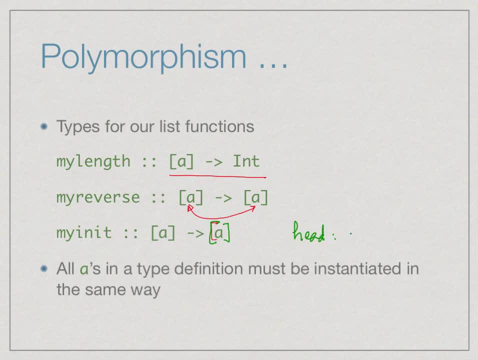 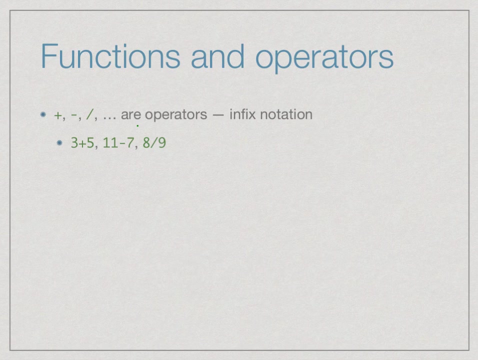 like head, for instance, then it would take a list of a and produce a single value of typing. so the important thing to note is that if I have a variable, then wherever it appears in the type, it must be instantiated by the same type. so let us digress a little bit about notation of operators and functions in Haskell. so we 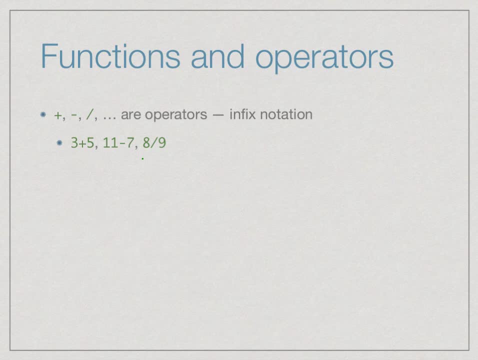 have seen arithmetic operators like plus, minus, divide. we also have, you know, boolean operators like or, and and. so we could have, you know, X and Y and so on. so these are operations which operate on two values, but we write them in this, in fixed notation, that is, we put the operation in between the arguments, right. 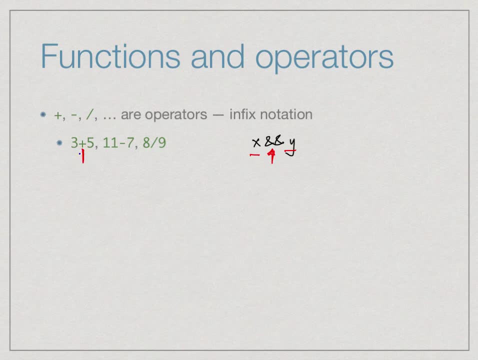 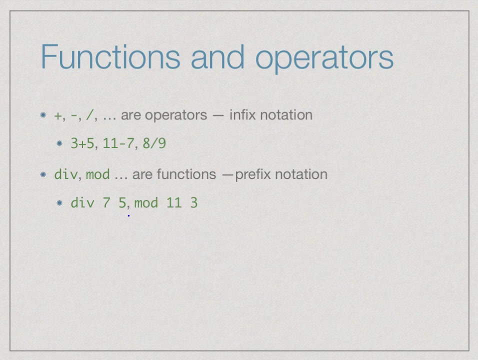 so we have two arguments and the operator comes in between. so the operator is, let's say, this is said to be in fix. on the other hand, we have seen functions which are predefined, like div and mod, which are written as functions. in other words, you write the name of the function and then you write the arguments. so this is what. 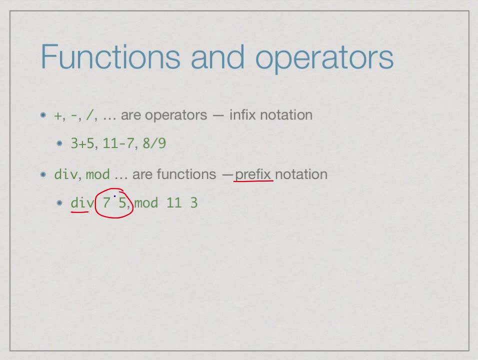 is called prefix notation because the function comes before the arguments. now sometimes you may want to switch between these two notations or two views. so in particular, we can take any binary operator defined and make it into a function just by putting round brackets around it, so the operator plus can be written as a. 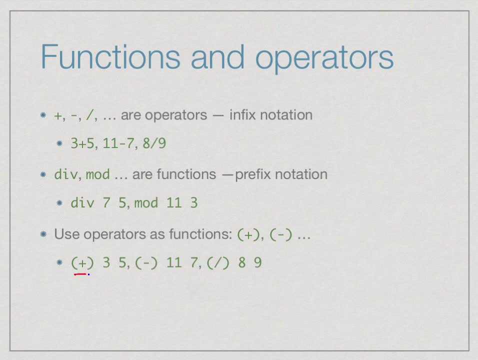 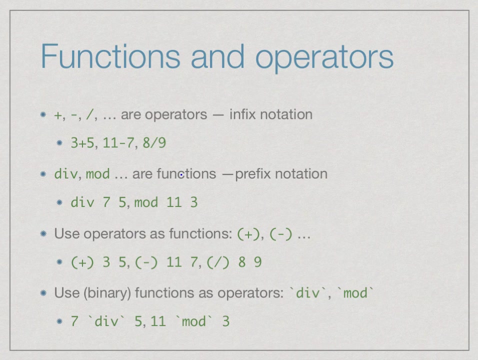 function by writing round bracket plus. so this expression plus three, five is exactly the same as three plus five and so on. so in this way we can use this notation to convert operators to functions, and we can also do the reverse, provided of course the function takes two arguments. 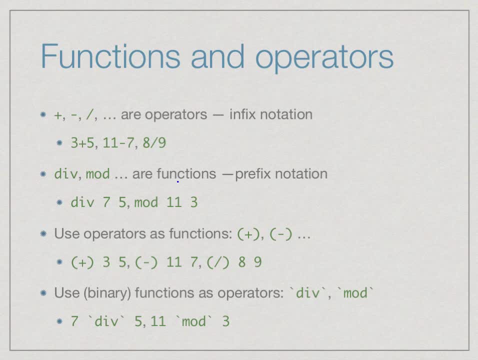 because otherwise it's not clear what it means to be imple in fix means it's between the two arguments. So if we have binary functions like div or mod, then we can use this reverse quote. This is the back quote key. This is not the normal apostrophe, but the back quote. 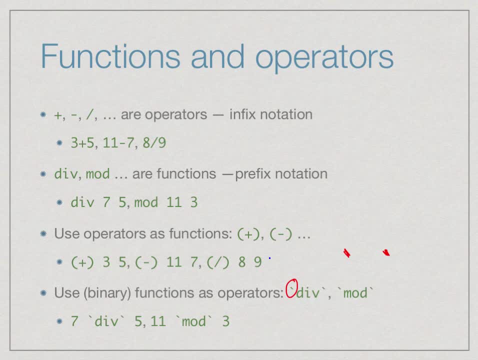 which you will find on your keyboard. So if we enclose the name of the function with these reverse quotes, then we can use them as operators. So if we want to say 11 mod 5 and not mod 11, 5, then we write 11 back quote mod 5.. So here we have written 7 div 5, 11 mod 3, and so on. 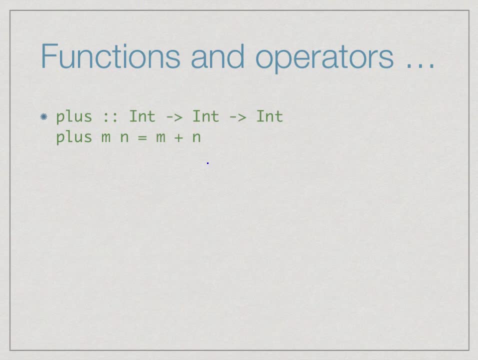 So this is useful in the sense that we have seen- Suppose we have written a function plus which takes two integers and adds them. What we saw is that, because of currying, plus actually consumes the arguments one at a time, So in an intermediate stage when it has consumed the first. 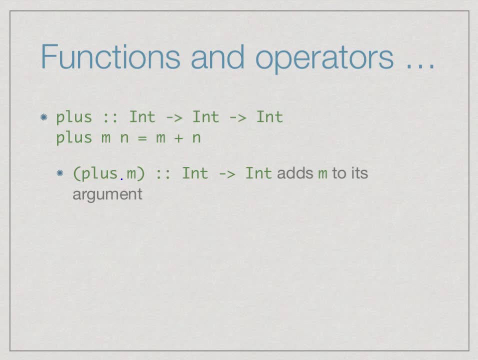 argument. we have a new function which we can write, called plus m, which actually takes whatever it takes as a second argument, namely the n, and it will add the two integers. So this is useful in the sense that we can add m to it. So m is now fixed. So in the same way we can think of this: 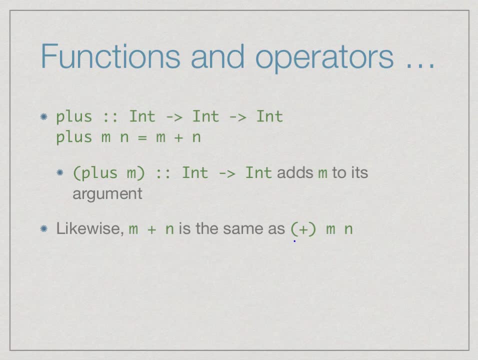 using the normal plus operator. So m plus n is the same as this round bracket plus m n. So this round bracket plus is a function which is exactly like the PLUS plus we wrote above, which takes two arguments, and if it takes one of them then it becomes the function plus m. So plus m adds m to. 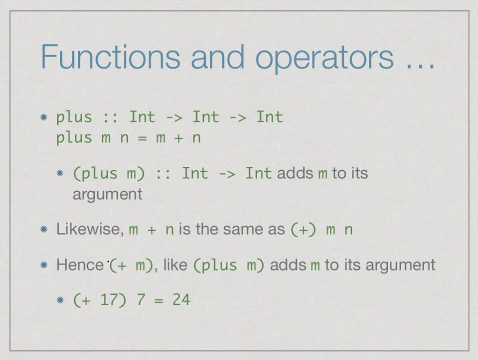 its argument. So you can try this out in the Haskell. So if you take something like plus 17 and you apply it to 7, then plus 17 will add 7 to 17 and give you 24.. So, using the fact that we can convert operators to functions by using the round bracket, 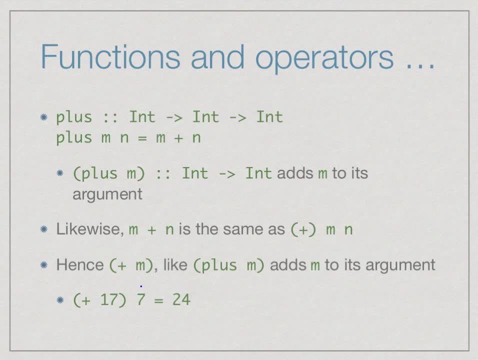 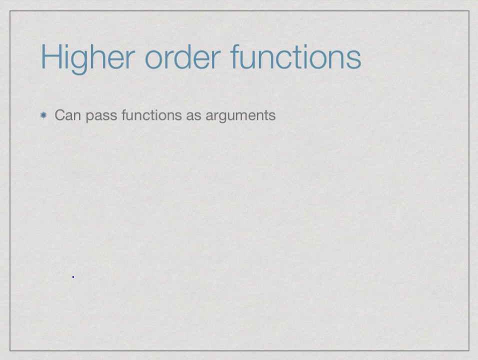 we can also get partially instantiated functions where one of the arguments has been fixed and use these when we manipulate functions in Haskell. Now, manipulating functions in Haskell takes us to this notion of a higher order function, So in Haskell there is no particular problem or specific thing that we need. 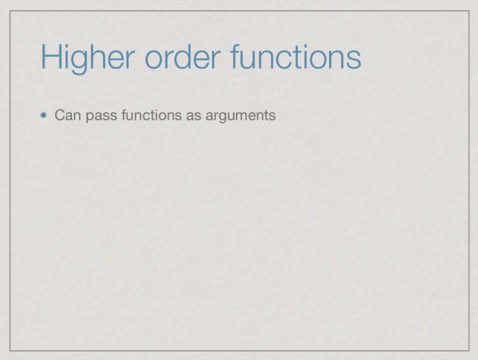 to do? to pass a function as an argument to another function. So here is the most obvious function we could write like this: So we can take a function called apply which takes two arguments and applies the first one to the second one, So it really reads the function as its first argument. 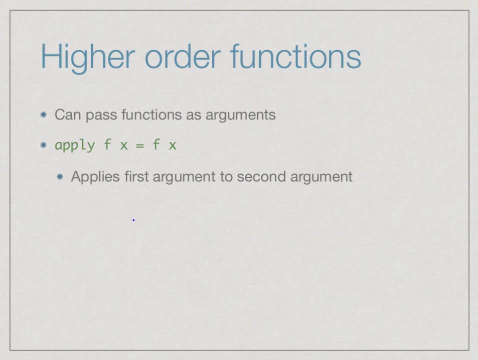 It reads a value as a second argument and applies the function it gets to the value it gets. So it just says: given f and given x return the value f of x. So here, for instance, if we say something like: apply the function plus 17 to 7, then this should reduce by the application of plus 17 to 7 to the value 24.. 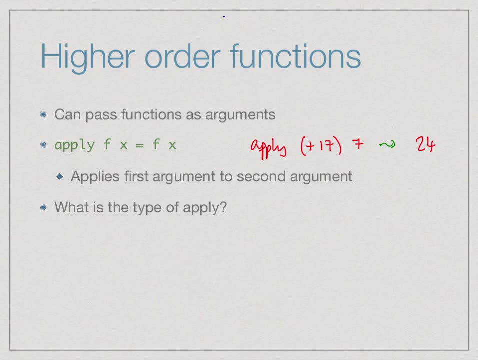 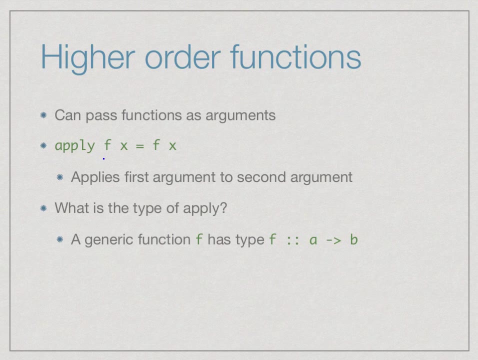 This is the intention. So what is the type of this function? Well, the first argument is a function, and we wanted to be possible to send all possible functions to apply. So if you make no assumption about the function, then it takes an input type and it takes an. 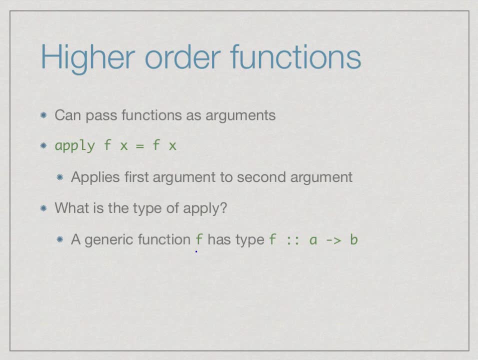 output type which may be different. So a generic function f has type from a to b where a and b are possibly different types. So there is no constraint. a and b may be the same type, may be different types. We do not constrain it in any way. 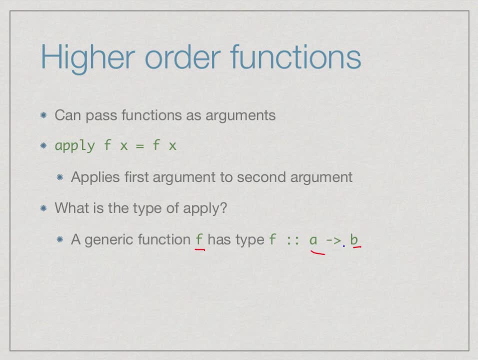 Now, given that f takes an input of type a and produces an output of type b, this constrains the type of x, because x is now going to be passed to f, So f takes a's, so x must be an a and the result must be a b. 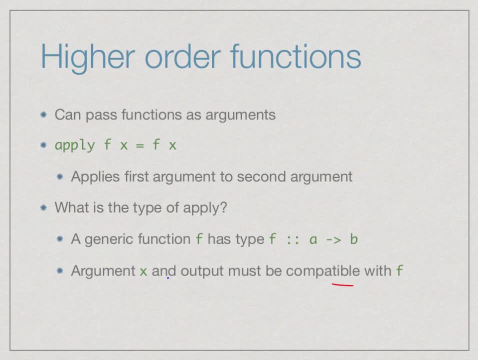 So the argument x and the output must be compatible with this choice. So this must be of type a and this must be of type b. So this gives us the following type. So this function, so this is not f but apply, So apply takes as its first argument. 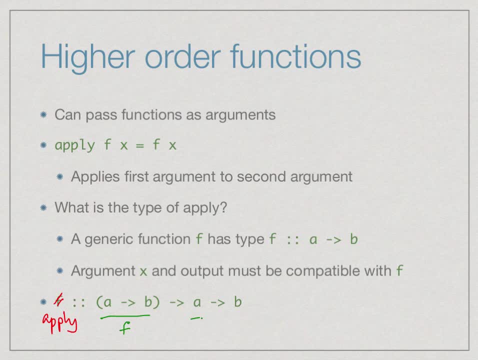 Some unknown function, f, and it takes as a second argument a value to be passed to this function and it produces an output which is the application of f to x which, because f has type a to b, this is of type b, So apply- has type from a function from a to b and an input of type a produce an output. 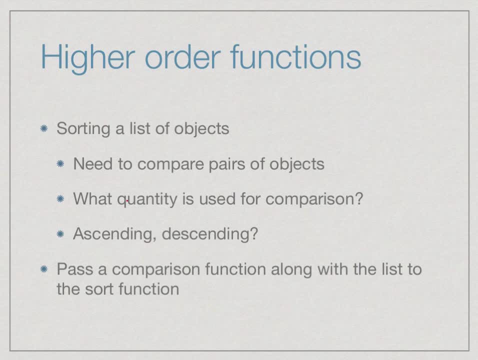 of type b, So higher order functions will turn out to be very useful. So here is a very familiar thing that you would have seen before. So suppose we want to sort a list of objects. At the heart of every sorting algorithm is a comparison between objects. 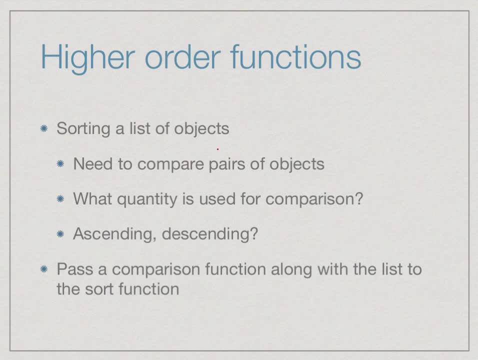 So we need to take pairs of objects and order them in the right way. So in some situations it might be important to know how to compare these objects. If we have pairs, then we use only one component, we use dictionary ordering and so on. 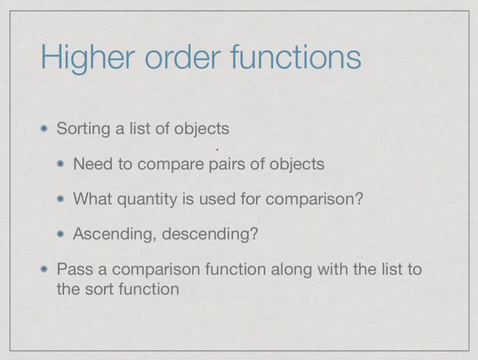 And also we might want to know in which direction to order them. Do we want to order them in ascending order, Descending order and so on? So, to be fully flexible, what we would like is that we have the sort function and it should take actually two inputs. 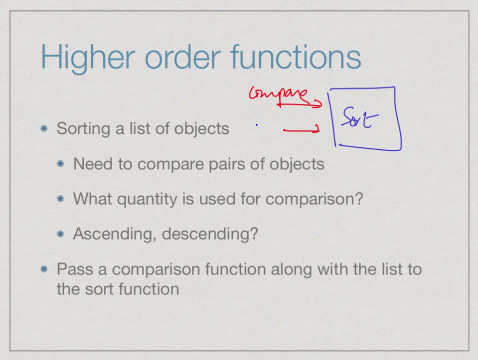 It should take the compare function and it should take the list And then use this compare function to sort this list according to the sorting algorithm. So by changing the compare function, for instance, we can make it go from ascending to descending and so on. So this is a natural situation in which we pass a function to another function.